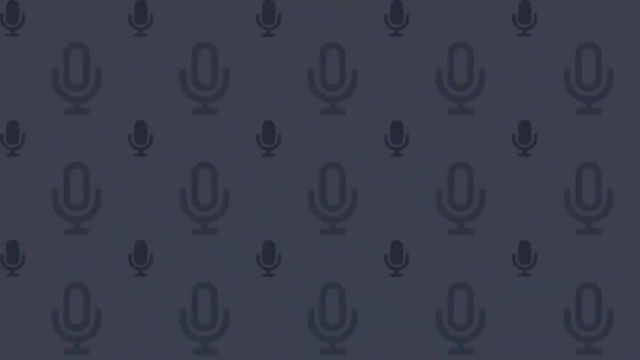 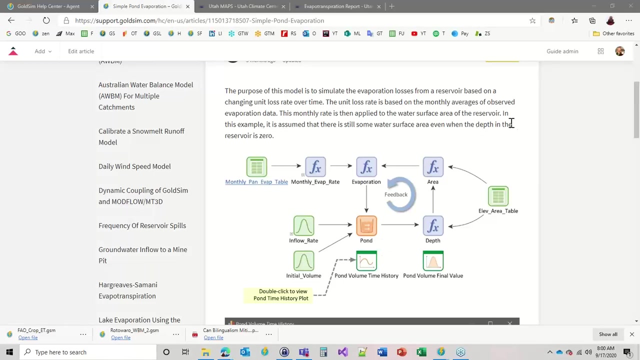 Today our webinar is on evaporation and evapotranspiration modeling this in GoldSim. This is part of the water management modeling series where I will be presenting- not just me, actually, me and others will be presenting weekly, every Thursday, both in the morning. 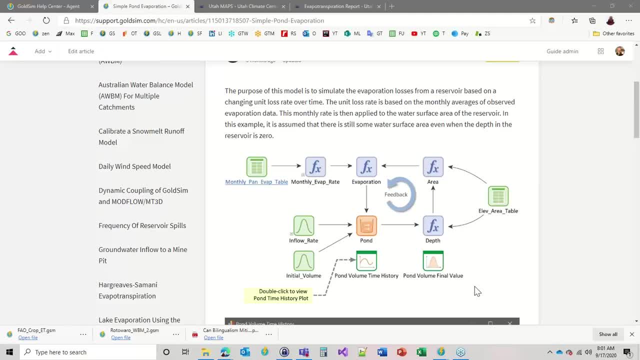 and in the late afternoon to provide a time that is convenient for, hopefully, all of our customers around the world, And these will be going all the way through to the end of November, And each of these webinars will, for the most part, build on previous ones. 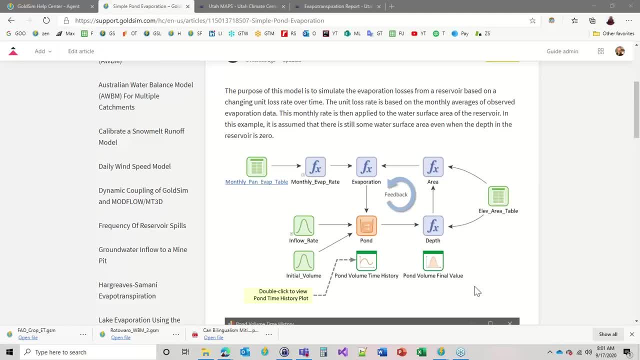 So it will help if you are able to attend each of these And if you cannot, we do record the presentation and post the video recording in our archive So you can always go back if you need to. So today, like I said, we'll be talking about evaporation and evapotranspiration. 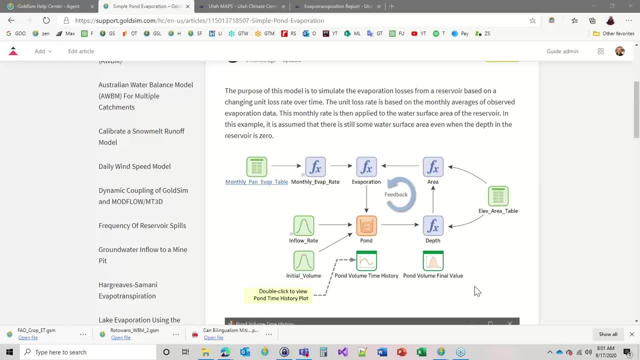 These models that I'll be showing you for the most part, are a function of temperature and possibly some other climate factors, But it might be It might be that you don't need to use a model necessarily to calculate these. Perhaps you could just reference measured data. 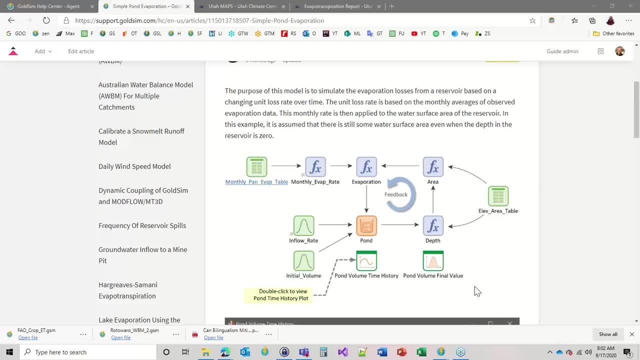 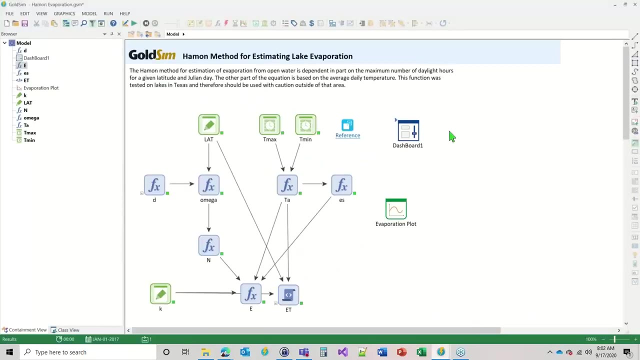 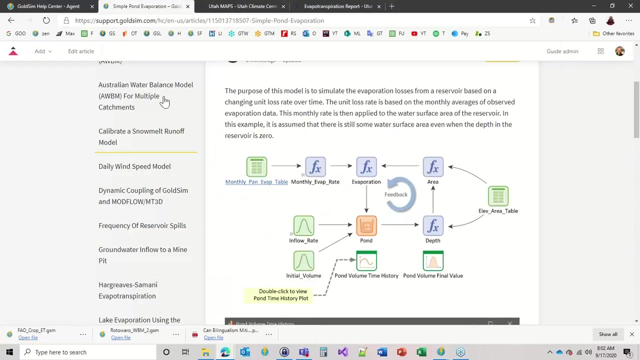 So I will talk about that as well. All right, So what we let's see. what I want to start with is a simple model, But before I go there, let me just talk a little bit about the data. So I'm going to back to website here. 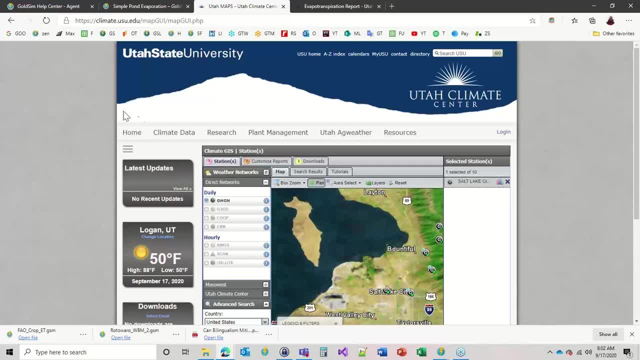 Now, this is just an example. This is: this is a site that's managed by a university in the state of Utah, Utah State University. It's a really good site and they have a lot of information here. In particular, you can download evapotranspiration like reference: evapotranspiration. 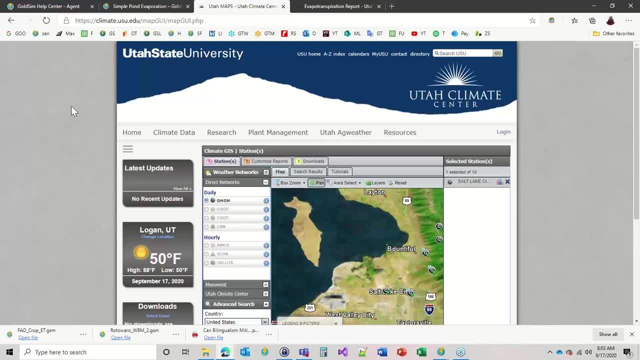 And I'll show you how to do that. Okay, And if if you're unfamiliar with that, just note that reference evapotranspiration can be used to derive the evapotranspiration or crop water requirement for specific crops, But it is kind of the baseline evapotranspiration that you can start with in order to calculate. 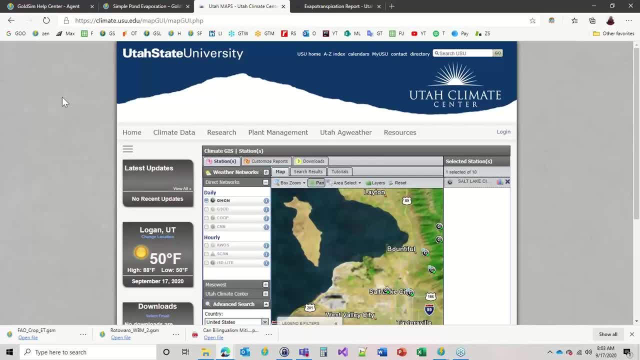 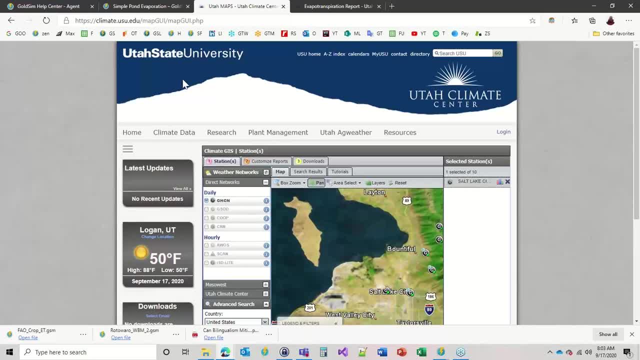 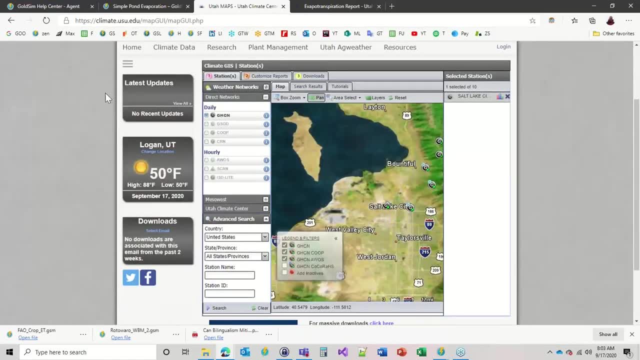 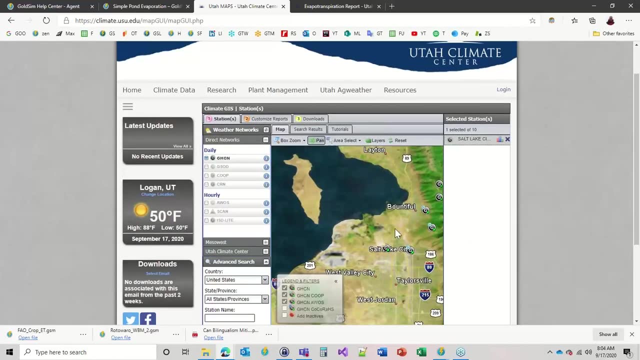 of water like a Lake, if you need to, from that information. So what you can do is you can go to this website here and you can see up here it's climateusuedu, And from here there is a, there is a way to browse various gauge stations and you 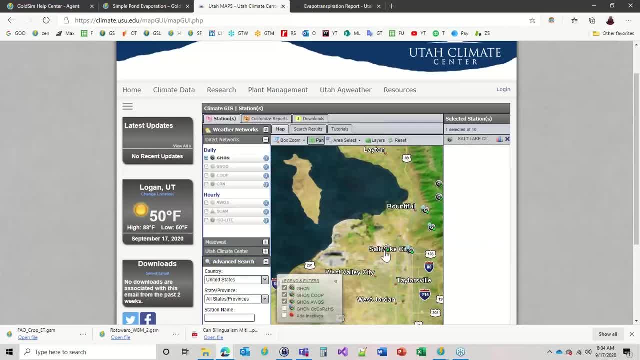 can look at the type, You can look at all the information about the environment, these different gauges, but when you click on it it will take you to the data. well, you have the option to go to the data. that is, if I click on it then there are. oh well, it was working earlier. 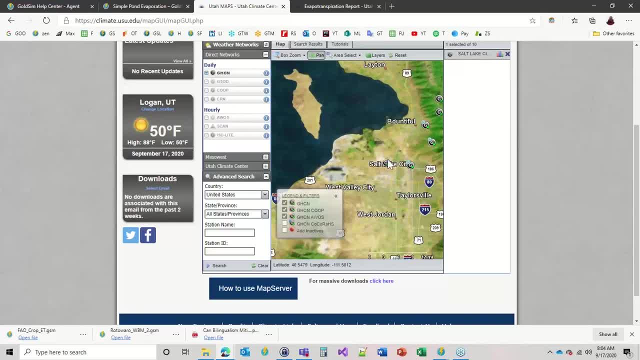 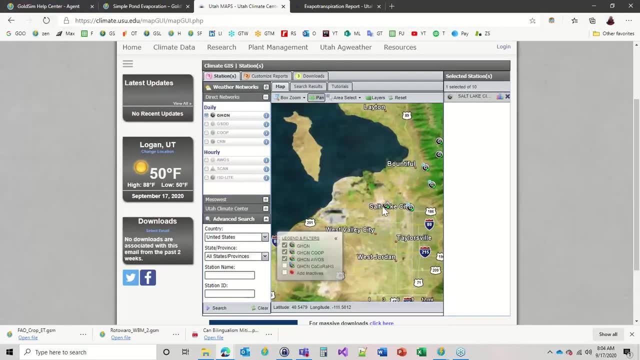 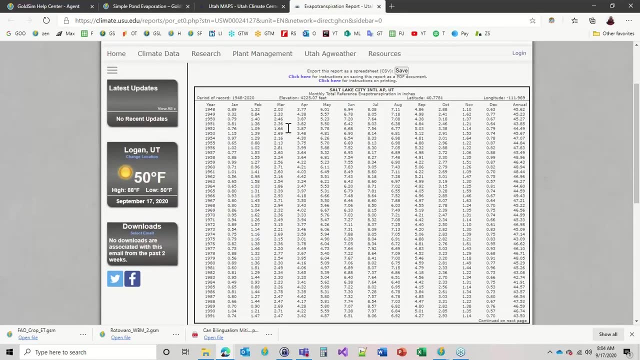 maybe I need to refresh the page, but anyway it maybe. if I refresh the page, then it will bring up a link that says you can look at the full report, which was just what I did, and then it takes me here. the only reason I'm showing you this is just because sometimes you don't need 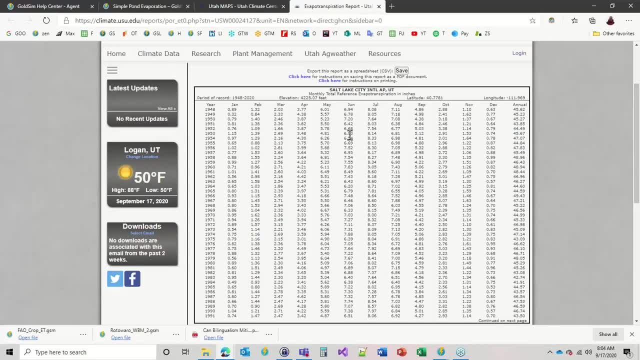 to model this kind of thing. sometimes you can just gather the data and and then just reference the data. so, for example, if we were looking at this, you can see it's formatted in a certain way that you can't just immediately start using in your model. you would have to. you know format. 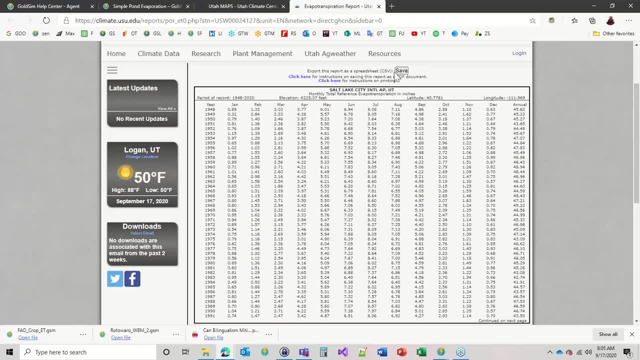 it in a certain way. but there is something here: you can download a CSV file and which you could save it as an excel file and have it automatically imported into gold sim. but probably best that you know you first review the information, make sure that it doesn't have any you. 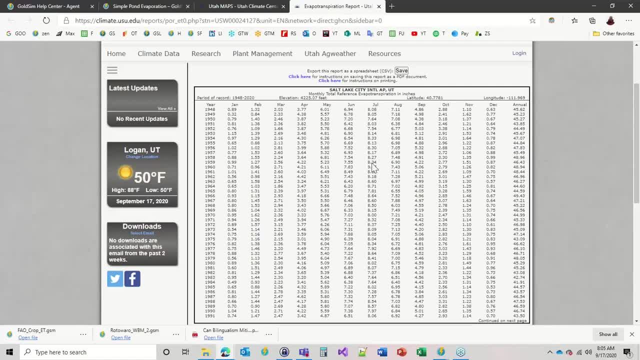 know blank values or non numeric values or in you know numbers that that don't work for this. all this data looks pretty good, but you just need to format it, put it into a time series, for example, and then you could use it in your model. this way now we did in the 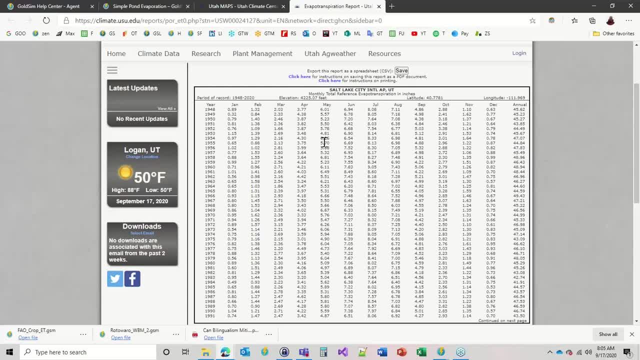 previous. in the two previous webinars, we talked about ways to take tabular data like this and then transform it, and also to interpolate values like, for example, monthly values, which is what we have here. you can put these into a daily time step model, for example, by interpolating between 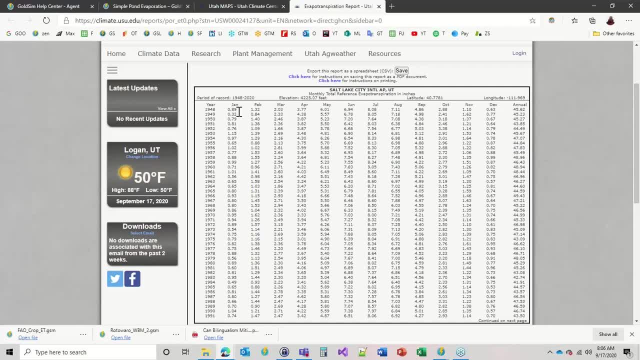 these values in various ways, which we talked about in the previous two webinars. so I'm not going to go back and rehash all of that, but just note that if you can get evapotranspiration or evaporation data or pan evaporation data from online and you're going to use that in your model, 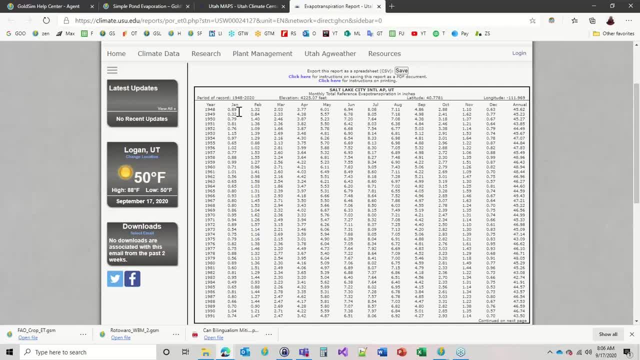 then just use the, the methods that we talked about before, to take tabular data and for you know, in whatever format that it's in, if you need to interpolate it or if you're just going to use constants over the month, or however you want to call it. but you can do that here and then you can. 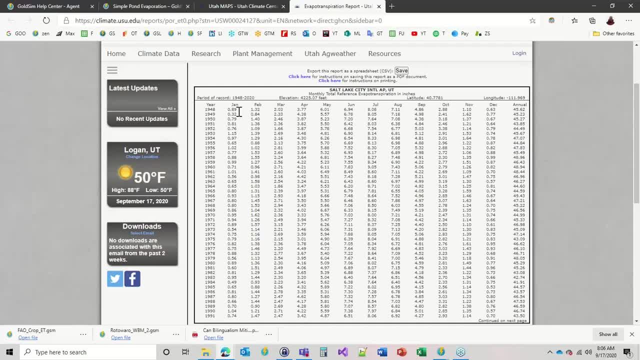 use the methods that we talked about previously, so I'm not going to spend time showing how you would do that here, just because it's it's the same. we'd be using the same methods that I showed you with precipitation, temperature, radiation and wind data, so very similar, okay. but I just wanted to. 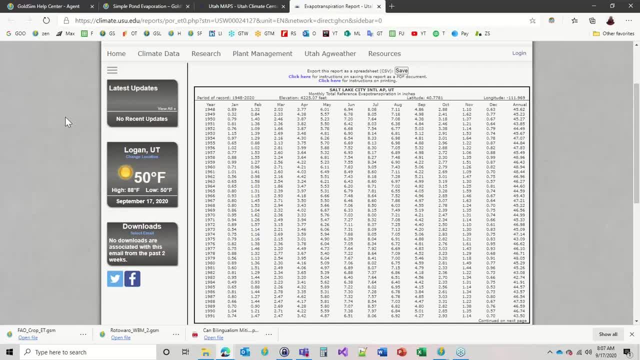 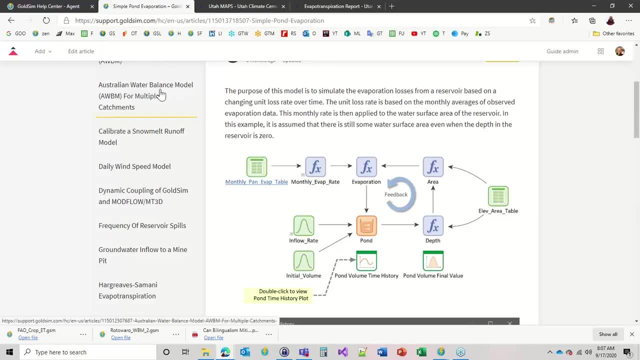 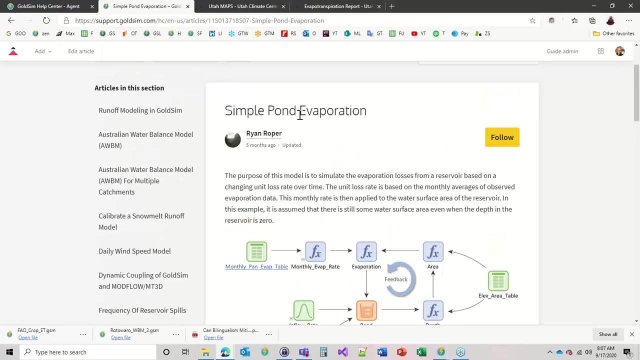 show you that, that this kind of information is accessible online for various locations. all right, so with that, then, you could do certain things like, for example, calculate the evaporation from from a reservoir by looking at the evaporation from the water surface of the Reservoir. here's: 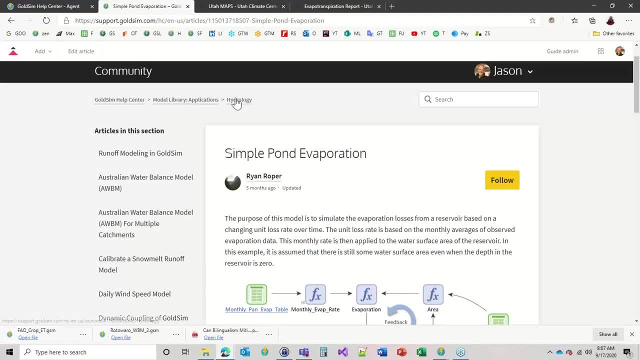 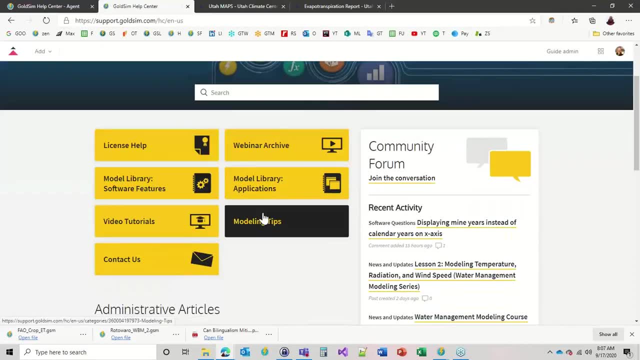 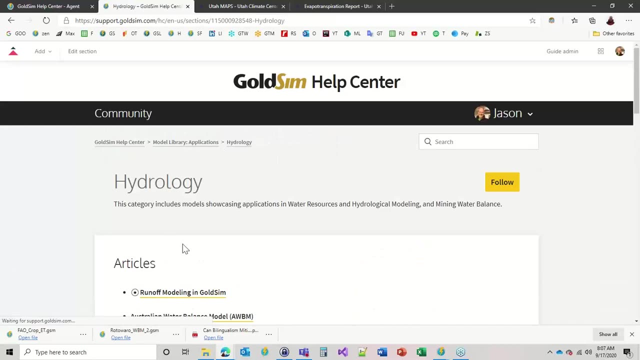 a simple pond evaporation model that you can get from our, from our library. now, just if you've not been to our library, just note it's our gold Sim help center. in here is a is a section called model library applications, and then in here it would be under hydrology. this is where you're going to be. 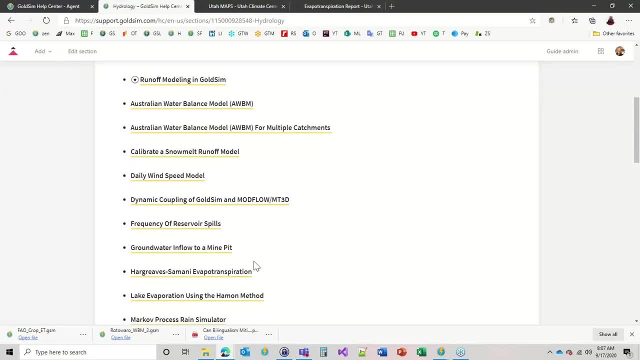 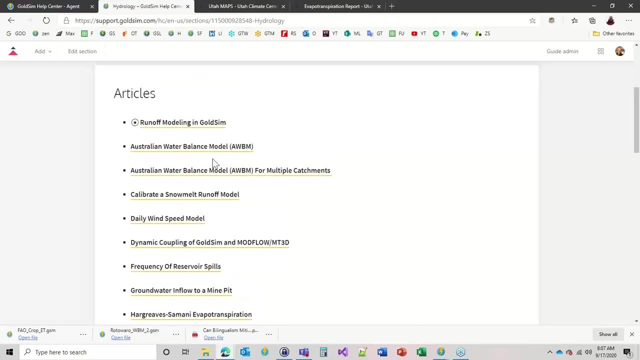 able to find all of the models that you're going to be able to use, and then in here you'll find anything related to evaporation, evapotranspiration, and we do have a few like this one here which I'll be showing you, and also this one. so, okay, so you can go here and and when you click on these, you 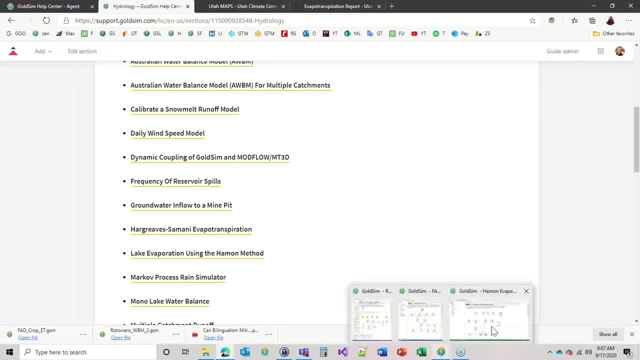 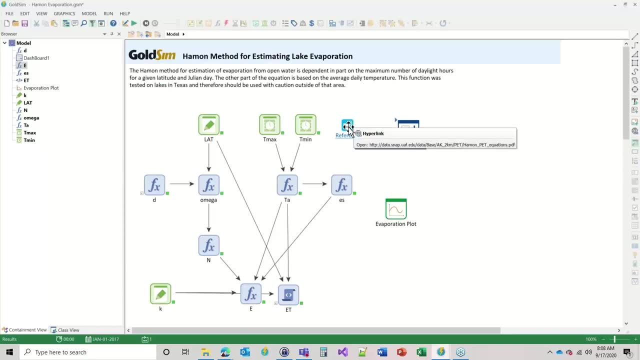 can download the model and use them as you might need. so the first model I want to show you is a pretty simple model called the Hammond method. there's a reference here. if you double click this, it'll take you to a website that talks about the pre-pandemic and the pre-pandemic and the 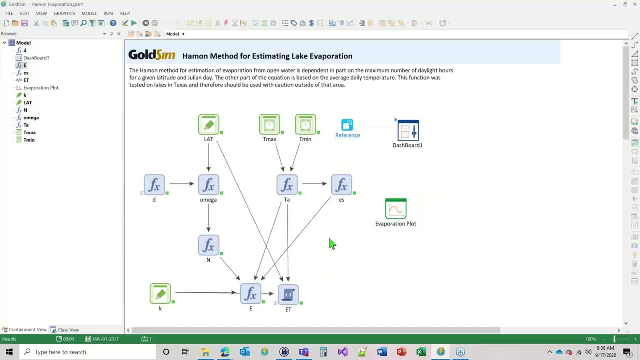 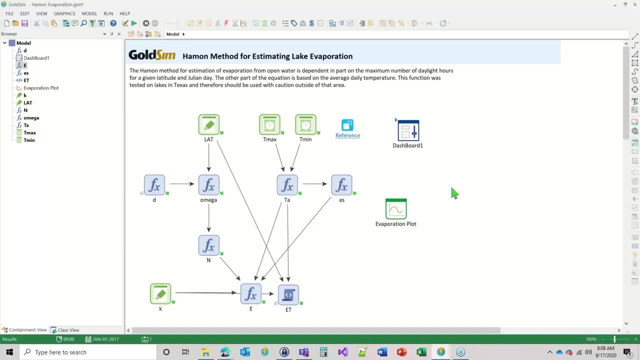 the physical process, but is just empirical. there is a coefficient that you can apply. don't get this K factor mixed up with crop coefficient, which is always denoted as K C. it's just called a proportionality coefficient, which is by definition a proportionality coefficient, which is by definition a proportionality coefficient. um and so apparently you could. 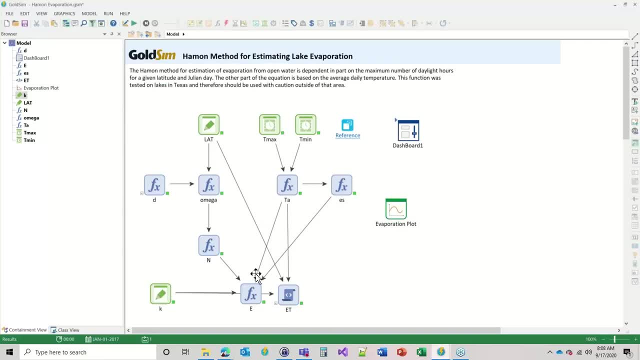 um, and so apparently you could perhaps make minor adjustments to this for calibration. um, it didn't talk about that a lot in the reference, but maybe you could, uh, go deeper into it and see. but what this model does is it calculates evaporation, and which can be applied. 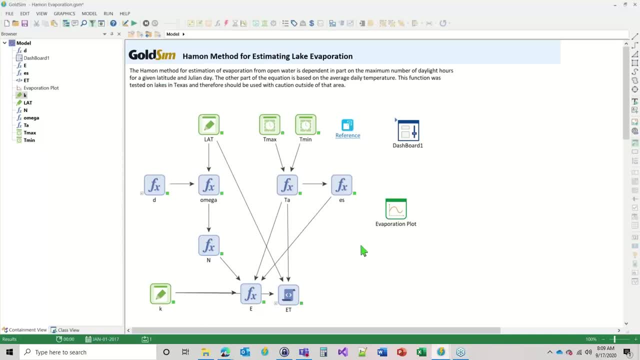 to a body of water as long as it is, um, not too shallow. if it's more shallow, then you might want to consider making an adjustment to it. but in addition to that, you can calculate evapotranspiration if you're looking at going into calculating, for example, water demands from certain types of of crops. but this is a very 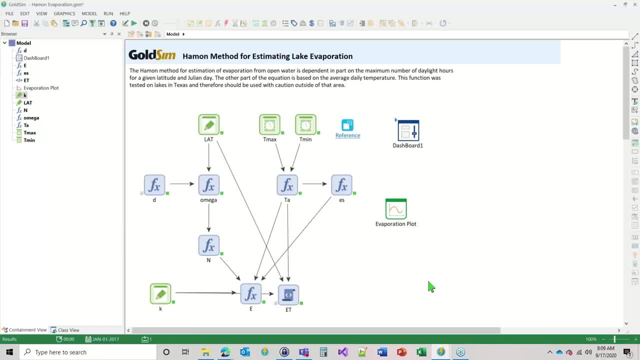 simple method and next I'll be showing you something that might be better if you're looking at calculating crop demands. but anyway, for for just a simple method that you want to calculate evaporation, this might be a good one, but just note that the main inputs to this model there are three. 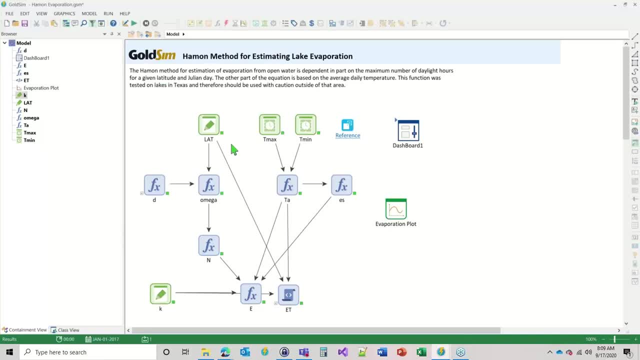 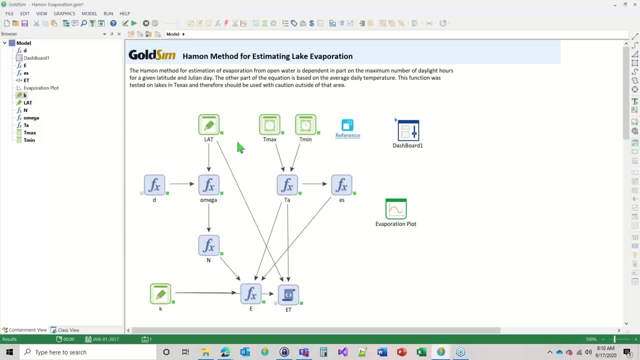 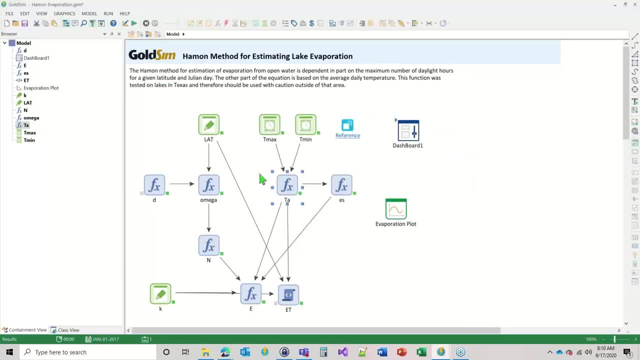 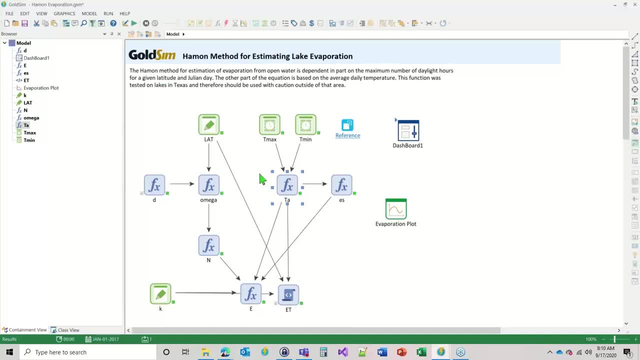 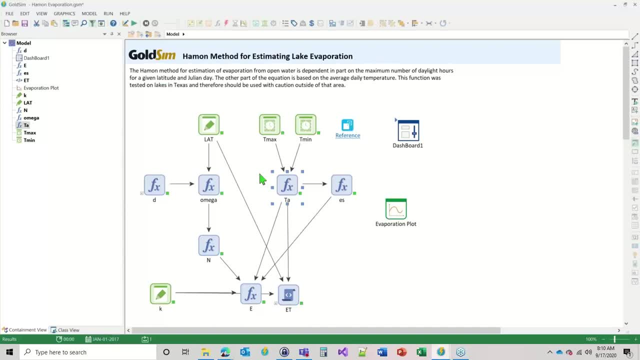 time steps than one day, but the data that I'm using is all for the most part- that's what a lot of these are used- is just one day time steps, so that's why I'm focusing on that. okay, If you look at the equation for evaporation, you can see it's pretty simple here. but one thing I just want to make note of is all of these functions that I'll be showing you for the most part, involve temperatures, and you have to be really careful with temperature data or the temperature units in GoldSim. 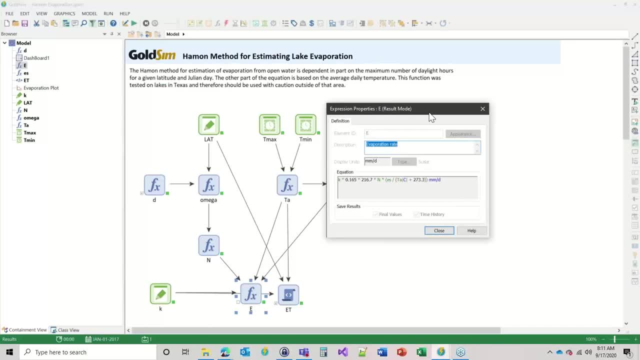 As you know, GoldSim is unit-aware, so all of the unit conversions are taking place for you in here. but with temperature you have to be a little bit careful, because there is a big difference between the temperature as a value versus temperature as a change or as a difference. 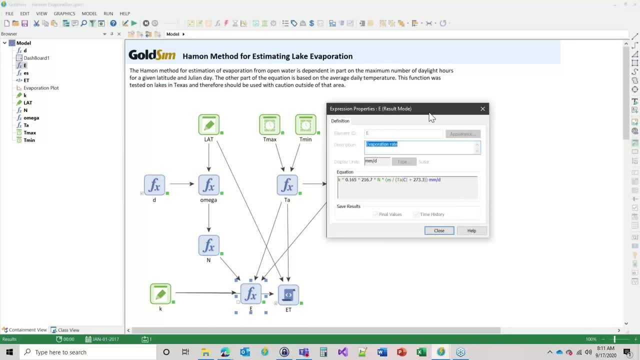 What I mean by that is, if you're trying to calculate, let's say, for example, the change in temperature over time, then that is a difference in temperature and that requires a totally different type of unit. and so let me just show you that difference. 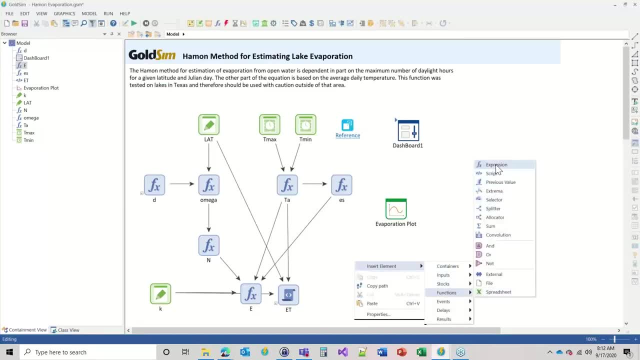 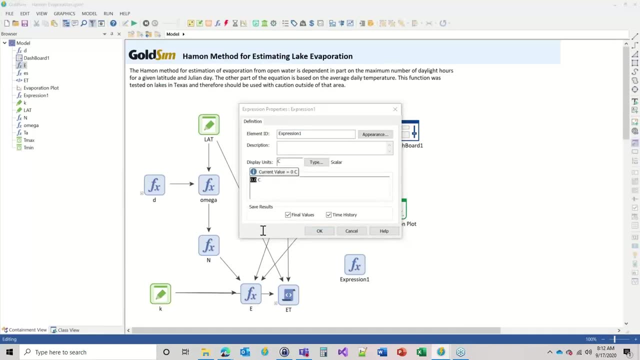 Let me just go to edit mode and I'm just going to create just a dummy expression here. but let's say we have temperature Celsius right here and I say, let's see, let's just say 20 degrees, Like that. 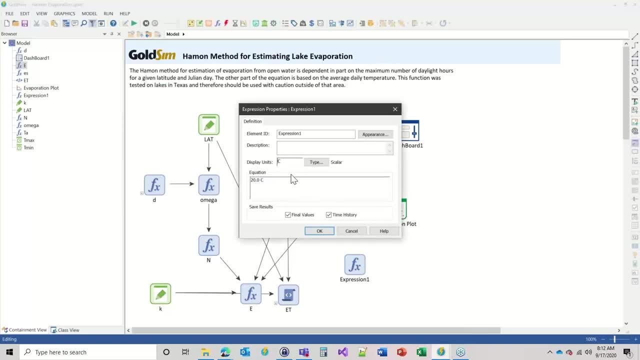 Okay. so if you're going to have a change, if you want to calculate the change in temperature, the difference, then what you actually want to use is Cdg, like that, Celsius degrees, and you'll see here that that is not converted to Celsius. 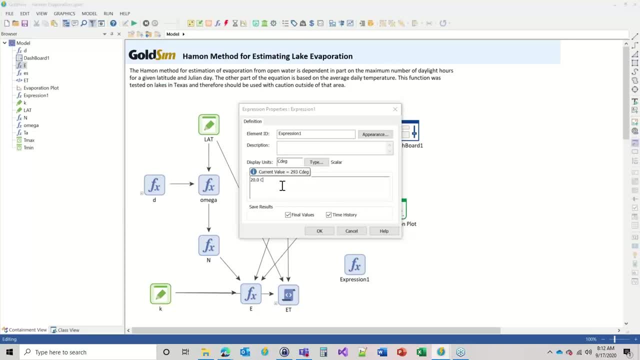 As you might have expected, it shows a very large number, and so that is Something to keep in mind here. you could have a conversion problem if you are not understanding the difference between these, or when you might need one versus the other. So just keep just as a rule of thumb, if you ever are looking at a difference in temperature between maybe two different temperatures, or if you're looking at a change in temperature. 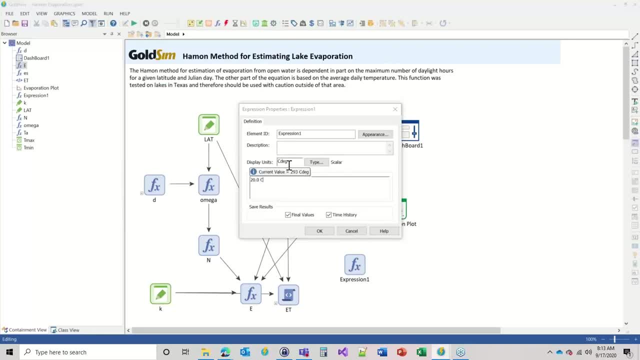 then you want to use the unit Cdg or F As an alternative to this. you could work in absolute, you could work with Kelvin And then you don't worry. you don't have to worry about this, this different type of unit. 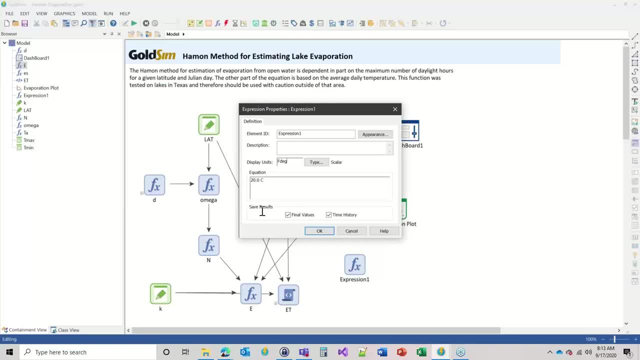 Another option is to just cast the units off and work with just unitless values, with an assumption that they are a certain unit, and then just go ahead and move on to it. Or if you have a couple needs, we can have a devAfter. do a way to eliminate the pendeterminate María, all right. 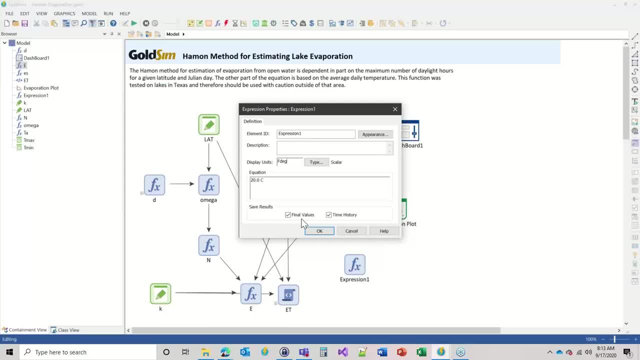 Or if you have a problem with November, there's also not much you can do. Then there's the presentation data. song輝ΟΞ is the��. we have to come up with another link there For other things: process test data, chords and all that. 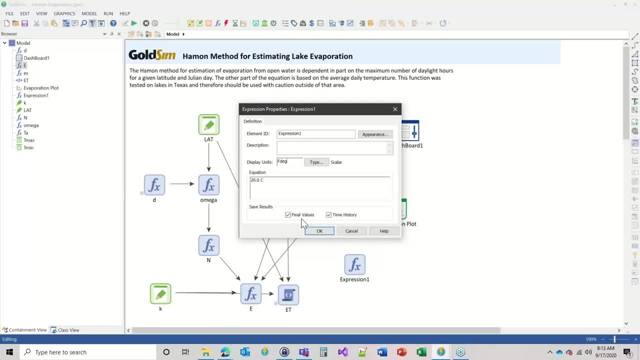 You can edit mode to see that, but there's a release of the key here. Okay, you guys ready, Right a unit and then at the end of your calculation, perhaps put the unit back on. So in some cases that's necessary, which I will show you. In some cases it's necessary because you might be working. 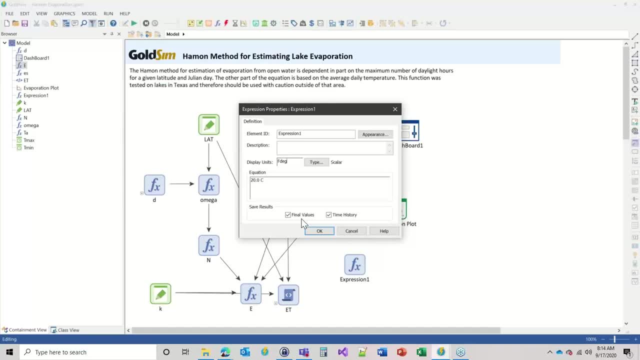 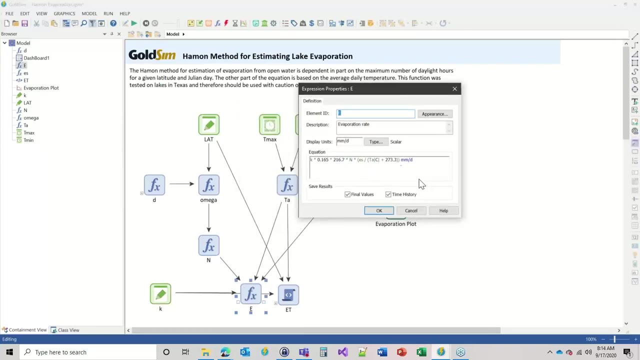 with an empirical equation that might raise something to the power, not to an integer power, for example, in which you could not use units anyway, And so you'd have to cast them off. So keep just be careful with units, And you'll see equations that sometimes look like this: 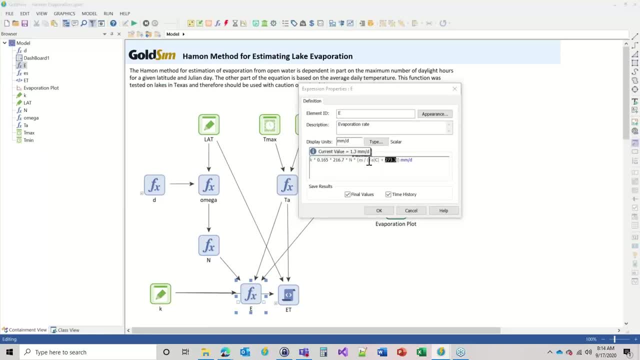 where you have a 273.3 in there. That kind of thing usually indicates that the well, actually that's not the exact number I'm thinking of. Let me back out of that again and I'll show you an example later where the value is actually intended to be in Kelvin, and it would be. 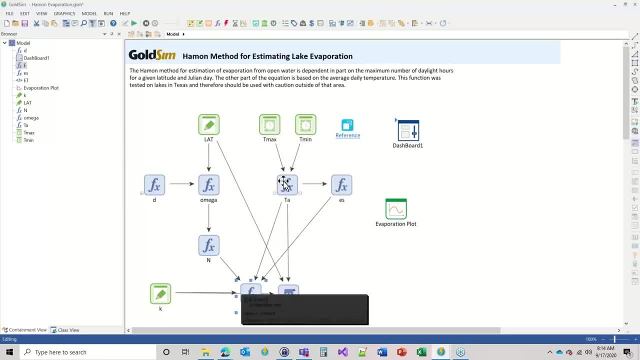 adding a number like that. But anyway, just keep that in mind, that just you need to be careful with the use of temperature units And we do have in our help documentation a discussion of that difference, which, by the way, you can always go to our help documentation just by clicking on help. 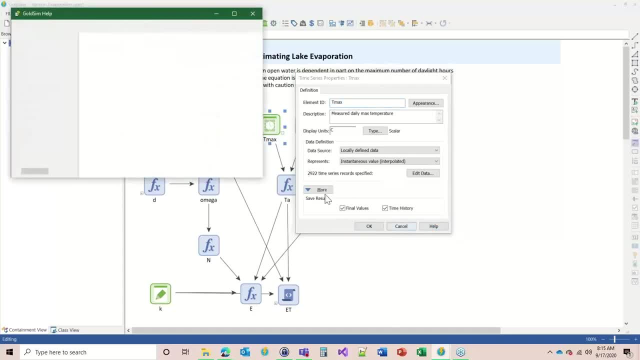 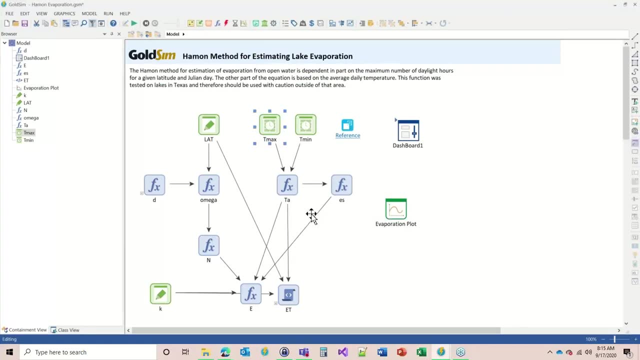 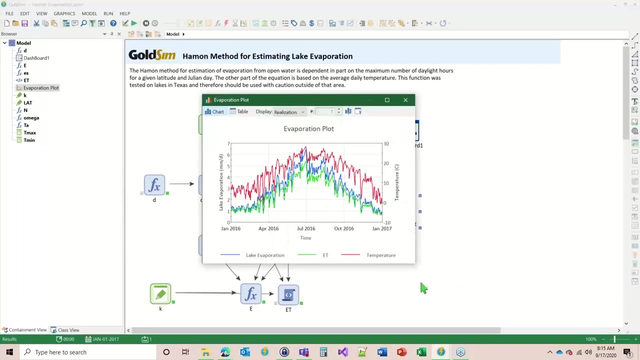 here or click on the question mark button up there and that will open our help System. Okay, So with this we run this model. Look at the plot, Then you can see here evaporation. Well, in this case we have evaporation. 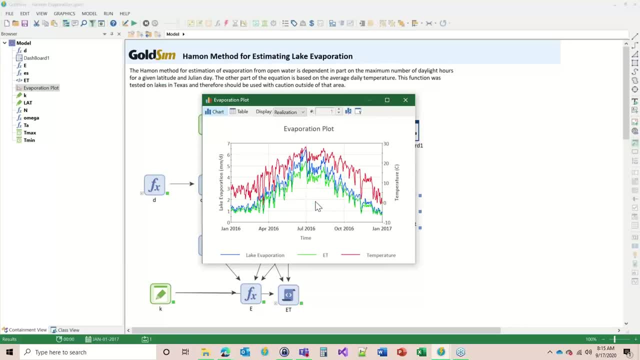 and that is also compared to ET evapotranspiration And you can see that it is that ET is slightly less than the lake Evaporation. And if you were to, if you had also, for example, if you had a pan coefficient. 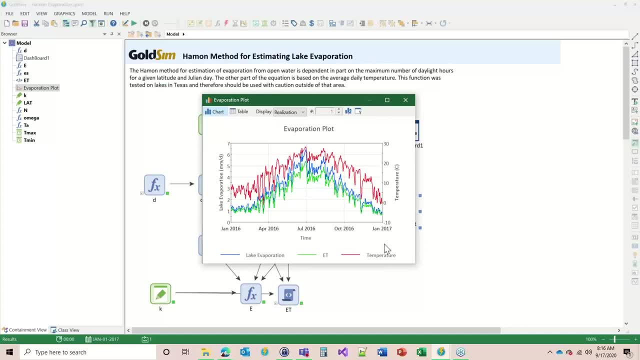 then that would also be slightly different here And you'd have to use some sort of parameter to convert between pan coefficient and- or sorry- pan evaporation and lake evaporation. I'll show you that in another model here, But you can see here that it is derived from temperature. 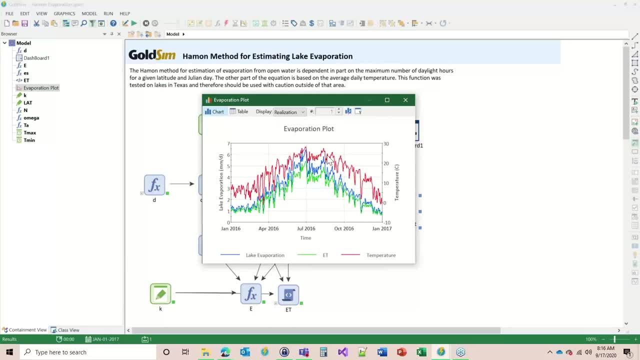 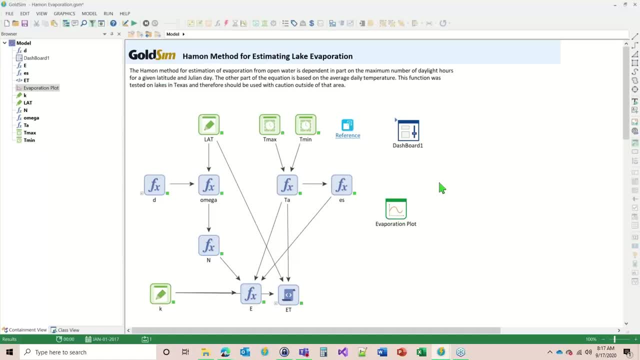 to evaporation, then you might want to consider using a different approach, Because, again, this is just an estimate, But let's look at how some of these simpler models might compare to measured data. So a similar model, a similar one to this, 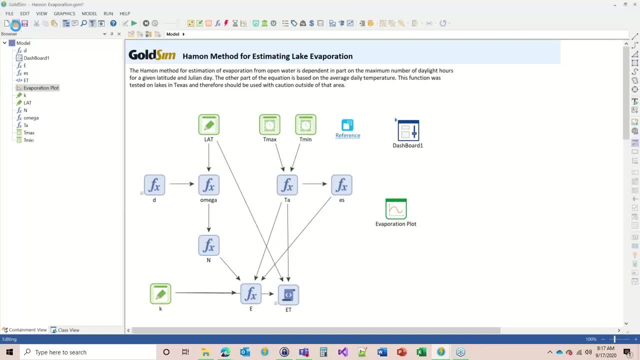 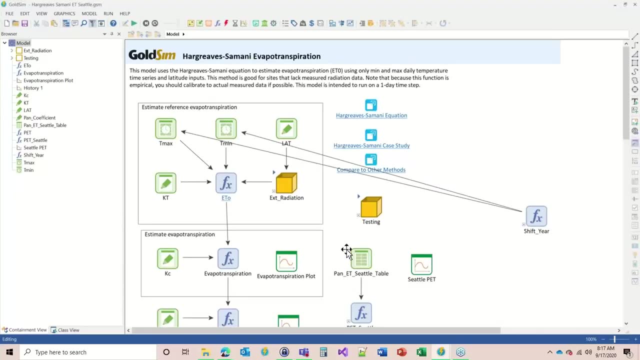 let's see if I already have it open. nope, okay. So a similar one to this is called Hargreaves-Samanai, And in this case I put in another element here so that we can use Monte Carlo simulation to sample the temperature time series. 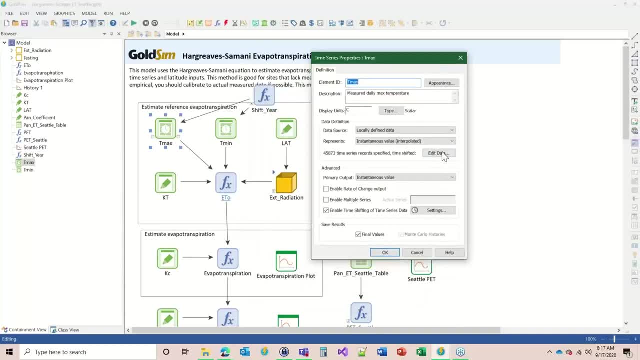 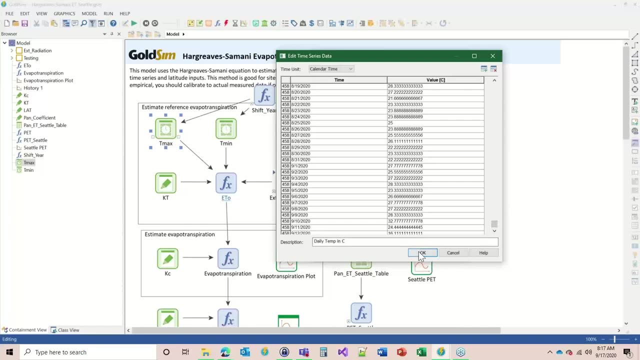 So if we look at the temperature here in this model it's measured temperature from 1894 all the way through 2020.. So it's a lot of information. Also, you can see that these values might look kind of strange. The reason for this is because the values 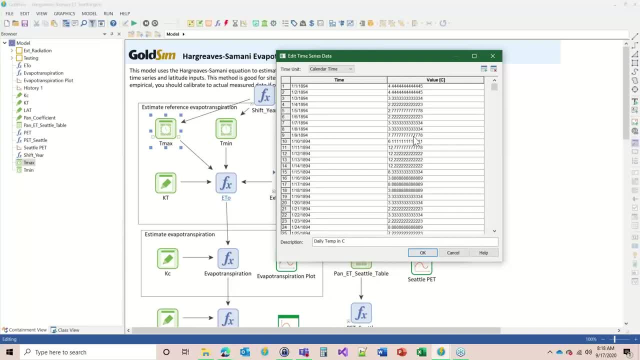 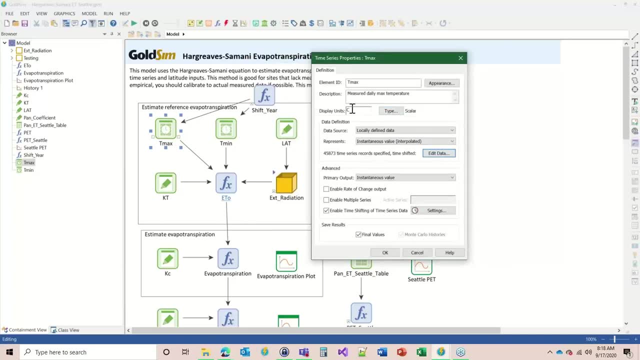 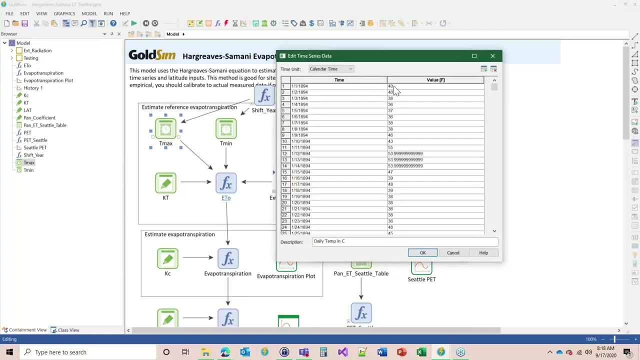 were converted from Fahrenheit and it was done immediately after pasting the values. So, for example, if I put in instead of Celsius, I put Fahrenheit here and then go back to edit data, then you can see these values were automatically converted. 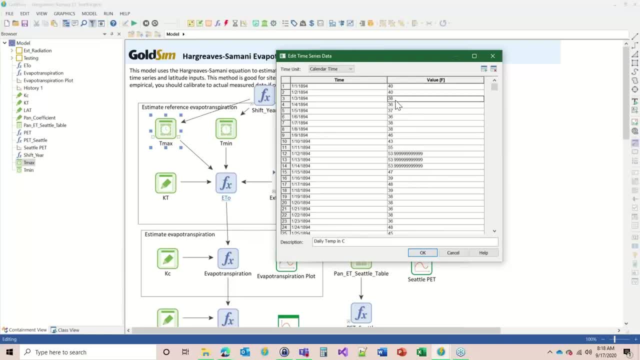 to Fahrenheit. So these are the values that were probably posted or downloaded from the web. In some cases there's going to be a slight a numerical error here. So you can see this was probably 54 when it came in. But all of these things can be taken care of simply if you. 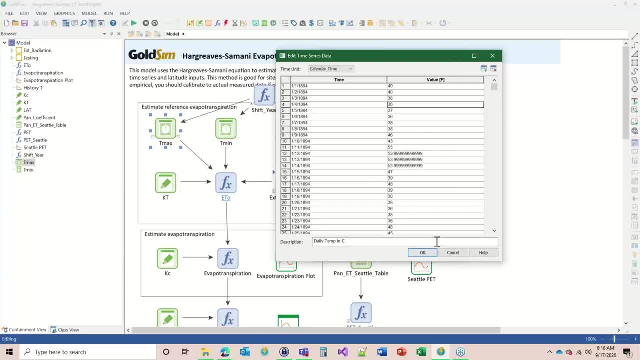 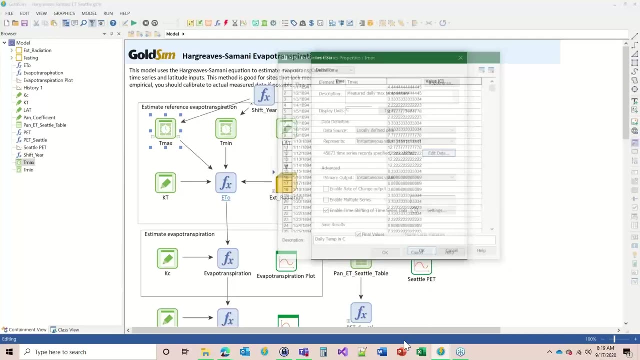 first convert them before bringing them into Gold Sim. But this really is not going to make any significant difference, obviously, to the result. but I'm going to put this back into Celsius So you can see that when it's in Celsius now converted again. okay. 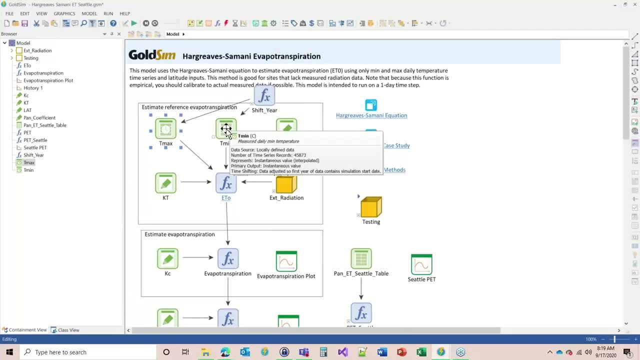 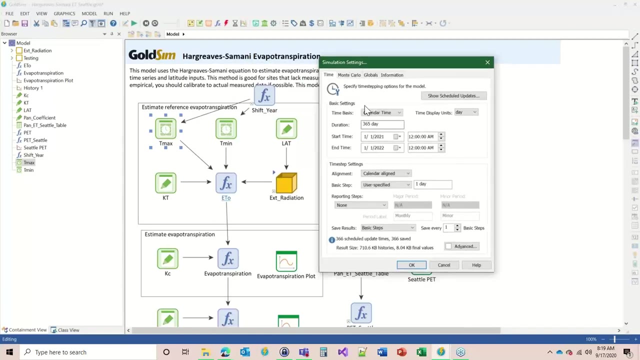 So we have TMACS and TMEN, quite a bit of data. We have enough data, in fact, that we could run many realizations and sample and get a good sampling of the entire time series series, which is what we were doing in this model. so if I go to simulation settings, you can see it's. 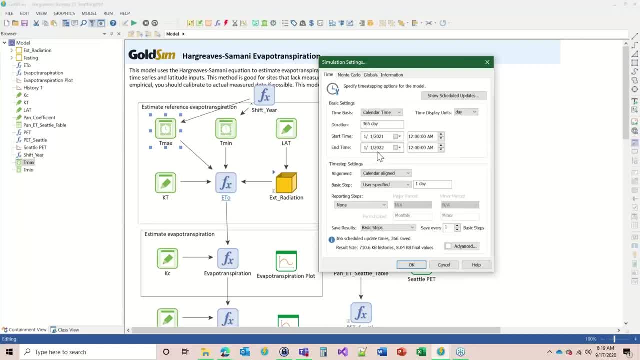 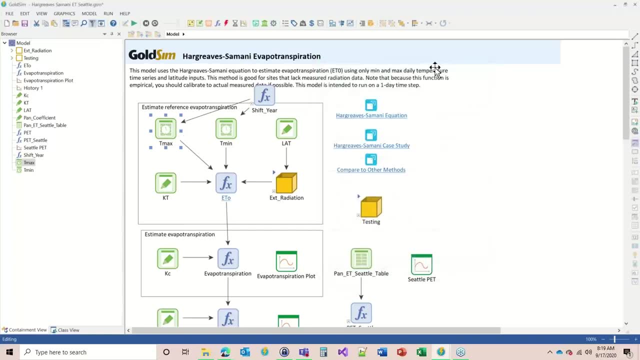 just running an arbitrary year, in this case the future, and then we go to Monte Carlo and you can see it's running 71 realizations, but in our case, because we have let me just check again when the start date, and so we can just check this, we could say 18 instead of doing the math in my head. I'm 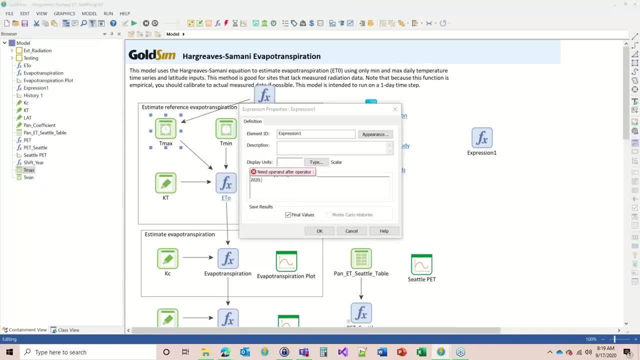 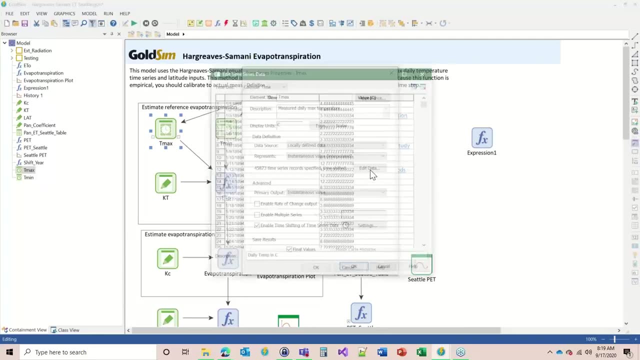 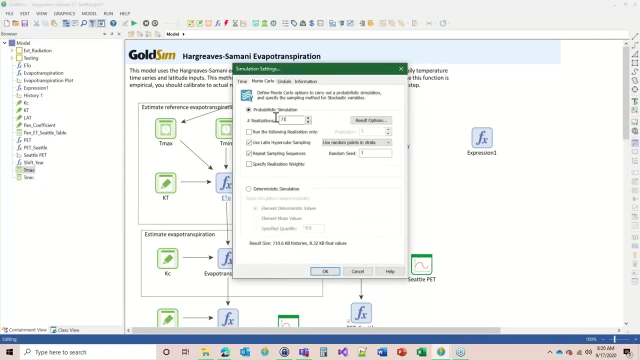 saying: let's see 2020 minus 1890. it was 1894, I can't even remember 126, so 18, okay, so about 126, I'm going to say 125 realizations. that's how, that's how many years we have of record there. 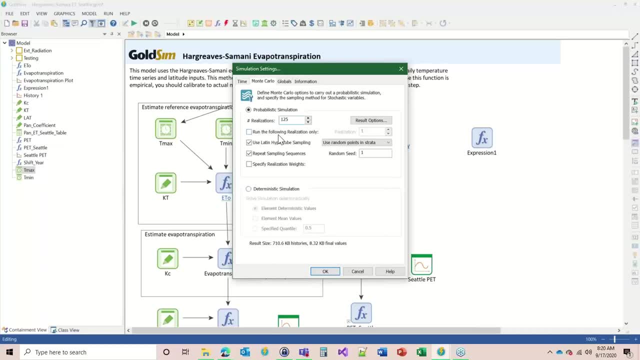 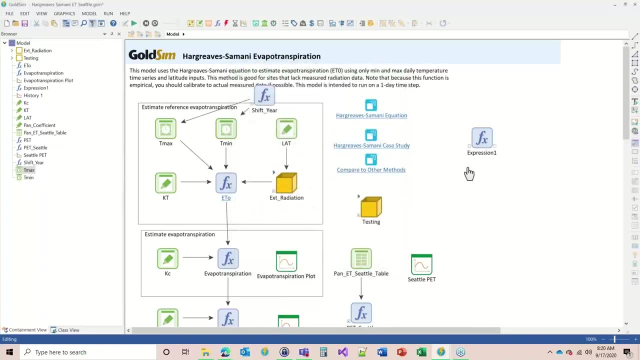 so we could run this model for 125 realizations, in which each realization represents a historic year. We could run more realizations, but that just means it's going to repeat or copy, It's going to resample the same year that it sampled before, which could be fine in this case. 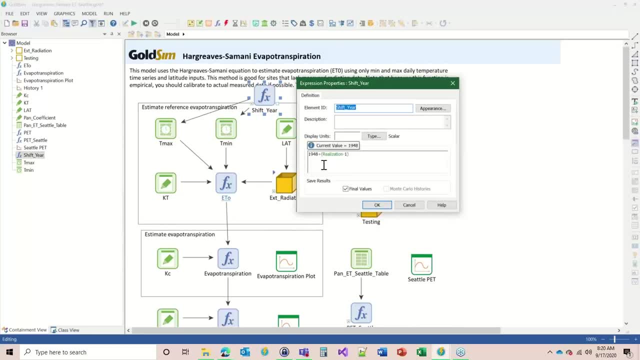 But the shift here is the key here. So what we do is we say: I want to incrementally walk through the historic record of temperature starting in 1948, but we don't actually need to do that. We could say 1894 and then add to that the realization, which always is just a counter, starting with one. 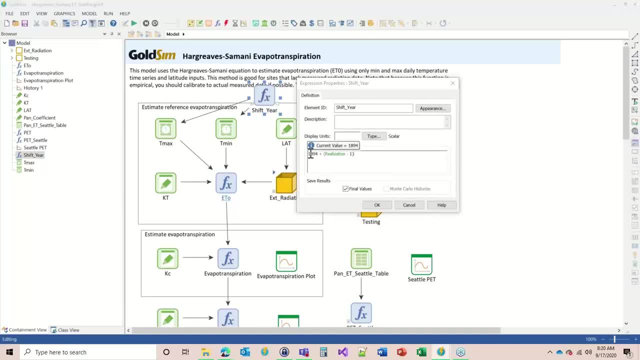 So you can see we have minus one. So it's starting with plus zero. That'll start us in 1894.. And then on the next realization, when this is two, 1895, and so on As you increment through all of the realizations in this model. I'm just going to move this a little bit here. 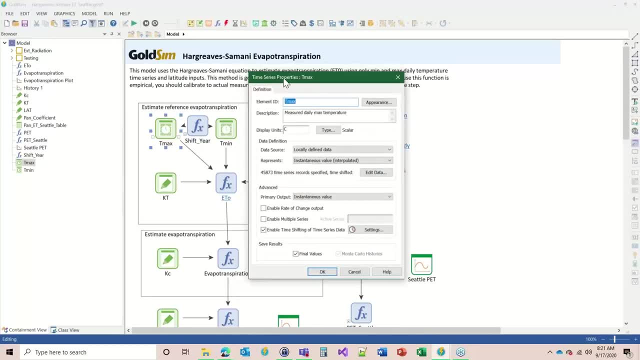 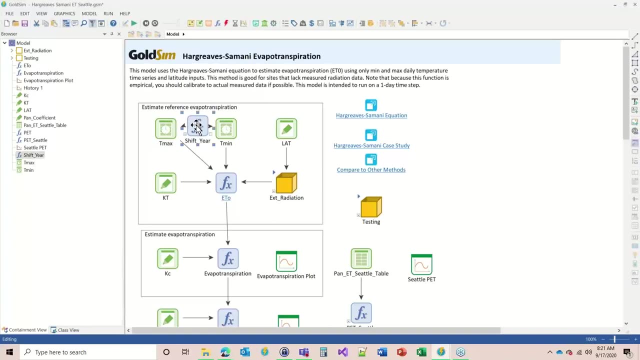 OK, so with that- And I talked about time shifting in previous webinars, but you can see the shift here is put there, And the reason we use this, this element here, is because then we can apply that to all of our time series throughout the model so that they're all aligned. 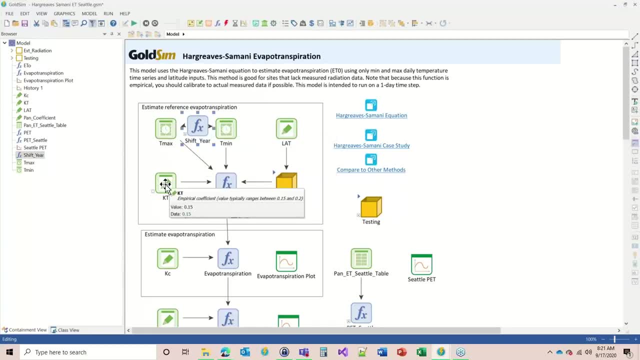 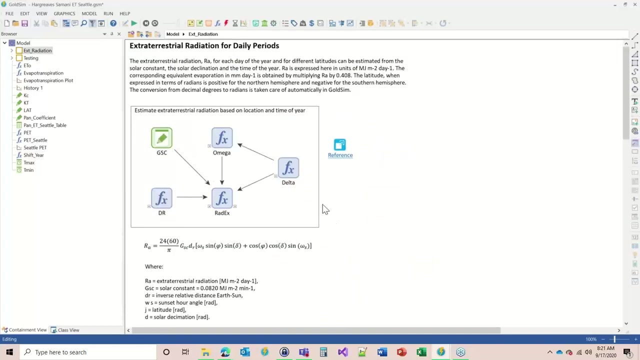 And that's what we want. We want all of our time series to be sampled incrementally, starting with the first year and then walking subsequently through as we go through each realization. Then, as we do that again, we also need to The latitude of the site and with that value then we can calculate the radiation. 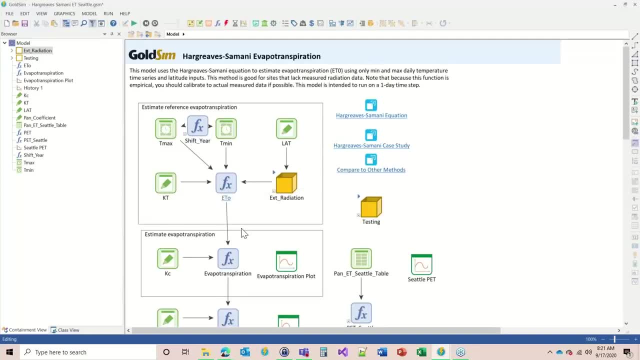 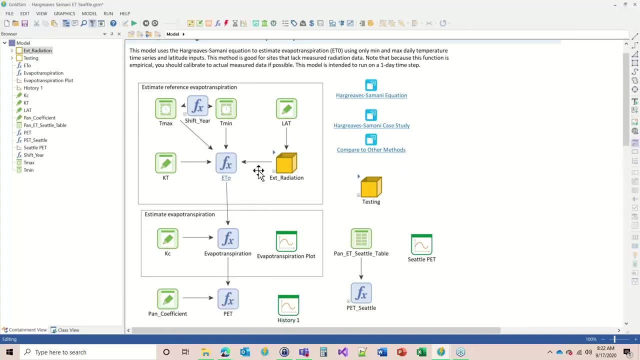 And from that calculate reference ET From that. And so you can see this is a little bit more detailed than the previous model I just showed you. The previous model did not have a calculation of radiation, so a little bit different. But as you work your way down through you can see that we. 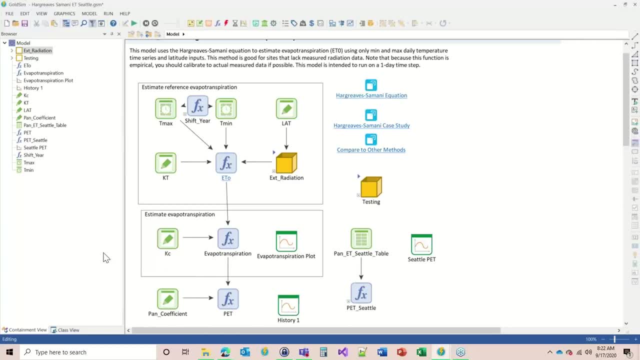 We end up with applying a crop coefficient in which you can then calculate evapotranspiration for a specific plan or crop. But you can also just back calculate the pan evapotranspiration if you wanted to. In this case I'm only doing it as a check. 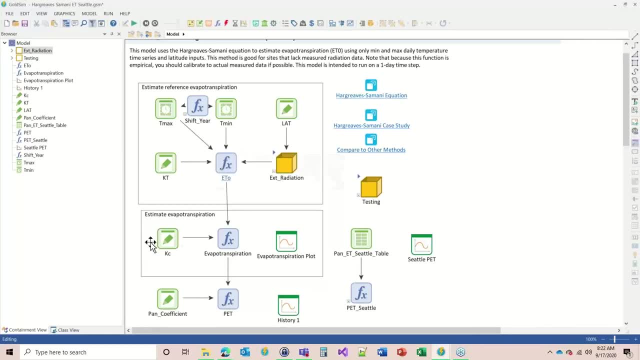 Now we could just apply that to the reference ET, obviously, But I have a KC value of one, So it doesn't matter. I could apply it to evapotranspiration over there and that'd be just fine. Anyway, what I have here is for this particular site. 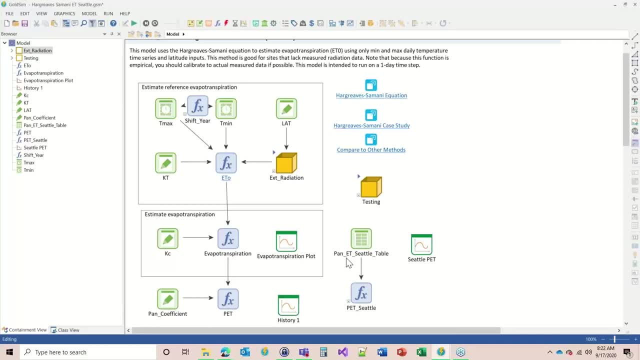 I have measured pan evaporation data for a particular location And now what I want to do is I want to essentially simulate the same output and then compare it. So if we run this model, Then look at a plot, Then this is just looking at one possibility. 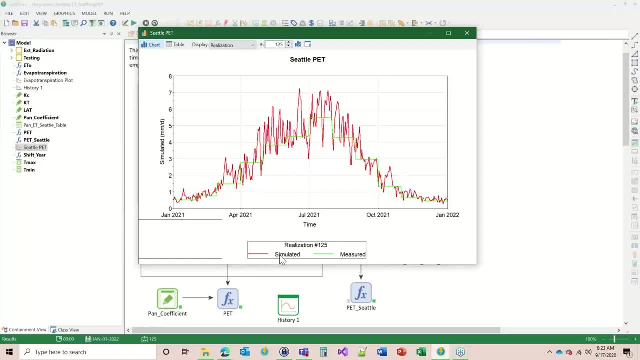 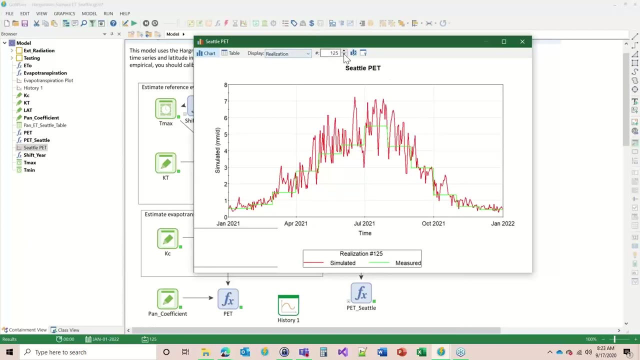 One realization you can see down here: Red. red is simulated, green is the measured, so the green is not changing in any of the realizations, It's just monthly measured evaporation. And so we can flip through some of these realizations and see how the simulated values are jumping up and down all over the place. 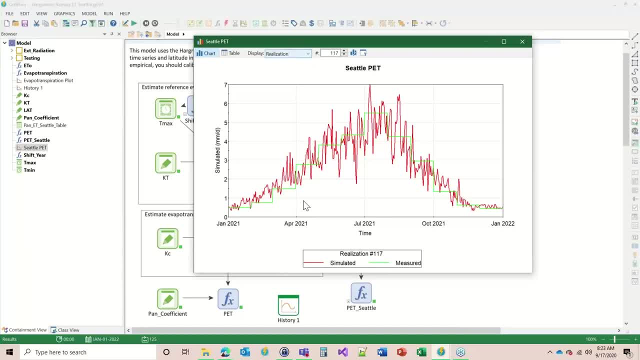 And it's really just because it is a function of the temperature. This general curve, the shape that we see in the red line, is a function of the site's latitude. If I change this to from realization to a statistic, they can see the comparison of how our simulated values on average relate to the measured evaporation rates. 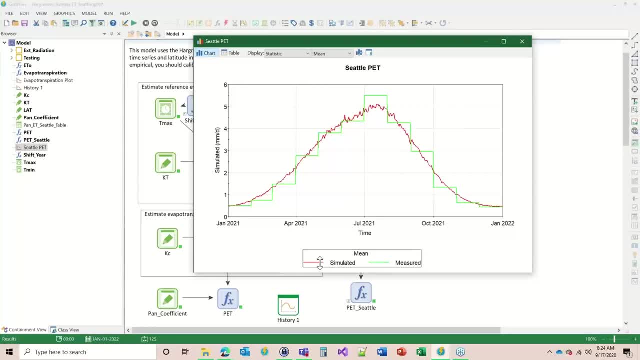 So It Looks like it's a pretty good fit. We would expect the values to kind of Go through the, the center points of these, these lines, and it's doing a pretty good job of that. It might, might, need to spike a little bit more in July to match a little better. 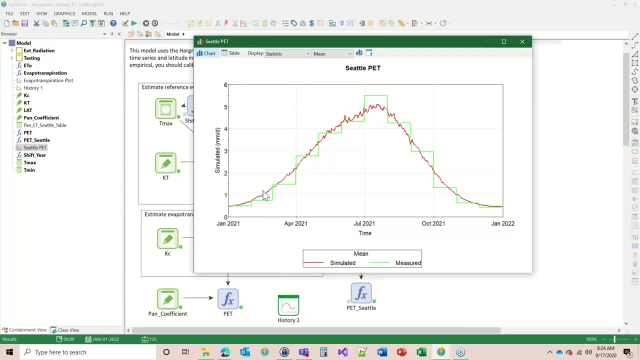 And, and also it might be going up a little fast here at the beginning of the year, But other than that it looks pretty good And so you can see This. this method, at least for this site, Under these assumptions, seems to seems to work pretty well. 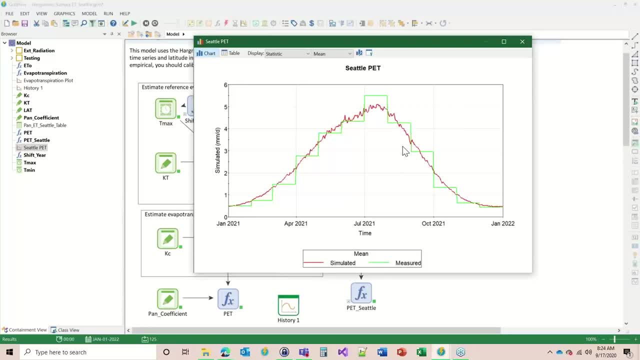 So if you're trying to calculate, for example, evaporation on on a water surface of a lake, then this might be- might be- a good method. Also, if you're looking at doing some simple calculations for a water balance that involves irrigating irrigating crops, then this- this might work too for that. 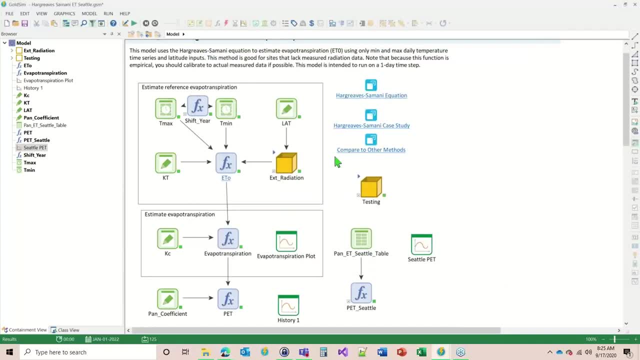 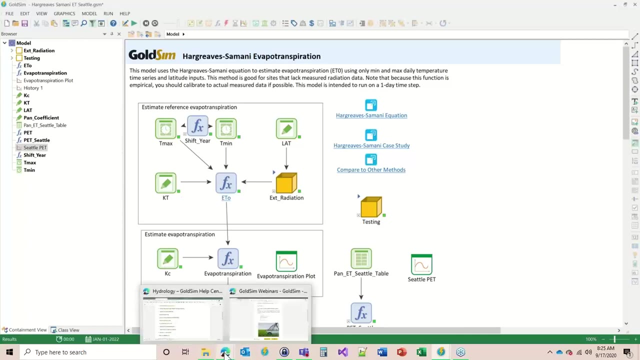 So You can also see. we have some links here for documentation of this method and also a case study. If you wanted to compare This, this model is available on our website. I'm pretty sure we saw that on there. There it is. 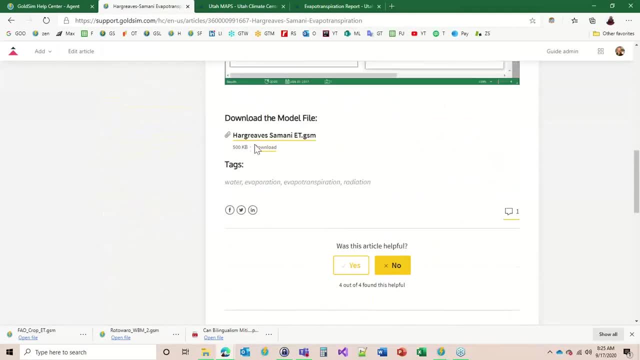 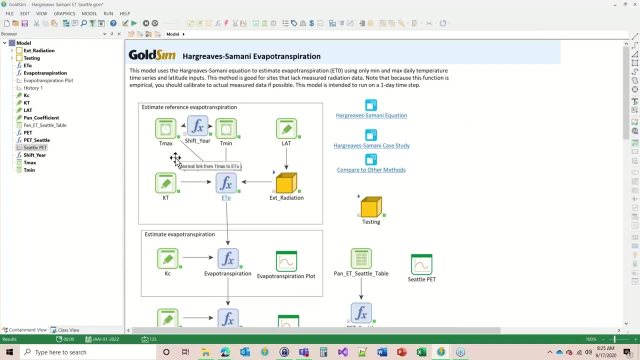 So if you go go here then, then you can read about it and also download the model and put it in. Okay, so just an empirical Method that is fairly straightforward, not requiring a lot of data, just temperature, but in this case not average temperature. it does require minute, daily min and max temperatures, but that's that. information should be pretty easy to obtain, maybe not for your exact site but maybe a location nearby, but still pretty straightforward as far as gathering that that kind of information. 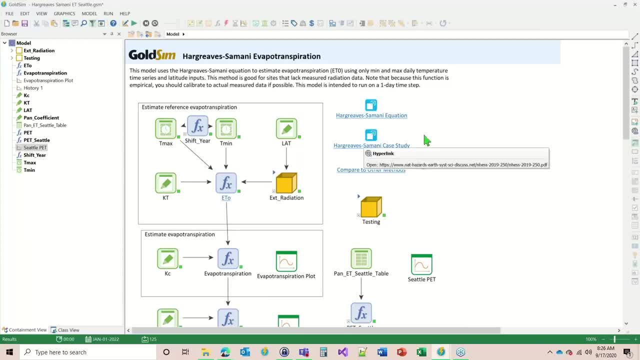 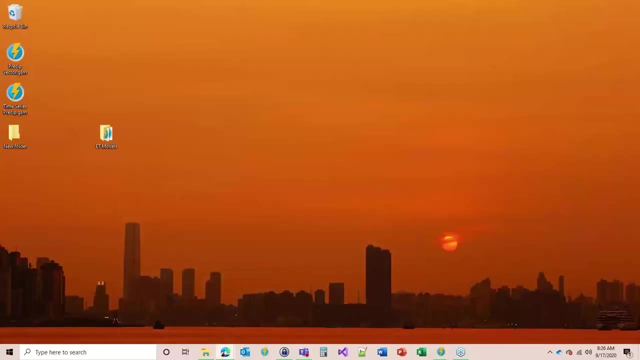 Okay, the next model I want to show you Is This Model I want to show you goes A bit deeper, and this is- this is a well known method, So let me You just close this, Okay, and this background pictures. 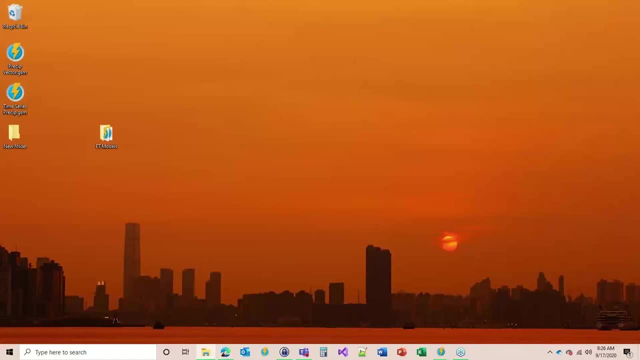 Pretty um Spot on for what's going on in Seattle right now with all of the smoke that we have. So I've been stuck, not only because of pandemic, stuck in the house, but also so stuck more because of the smoke. So it's been quite a week, All right. So the first thing I 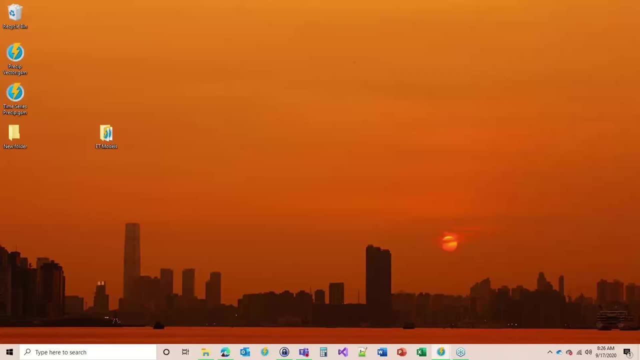 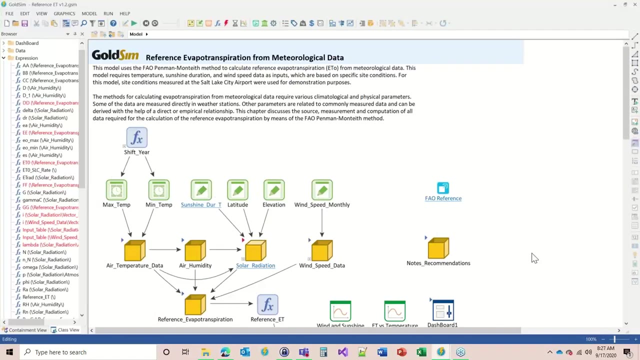 want to show you is calculating reference evapotranspiration using the FAO methodology, And I have a link here. This is a pretty famous methodology and there's really good documentation for it. This method uses more of a physical approach and I'll walk through some of those. 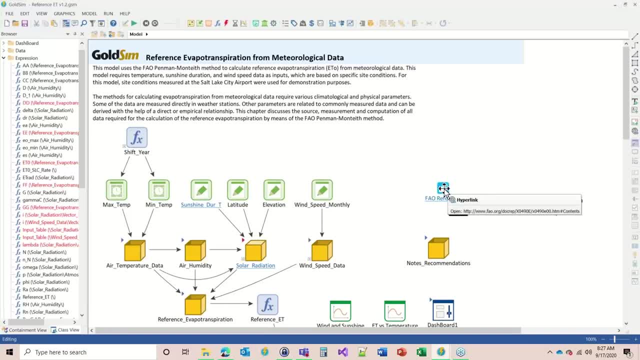 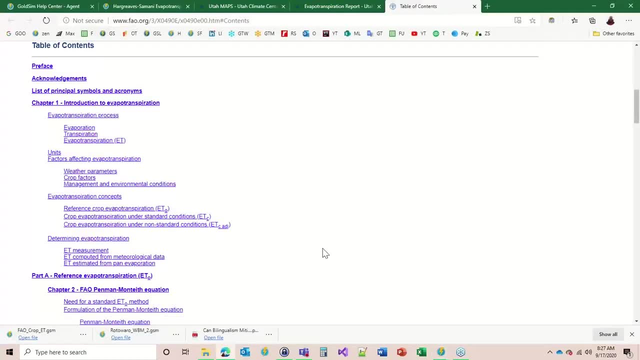 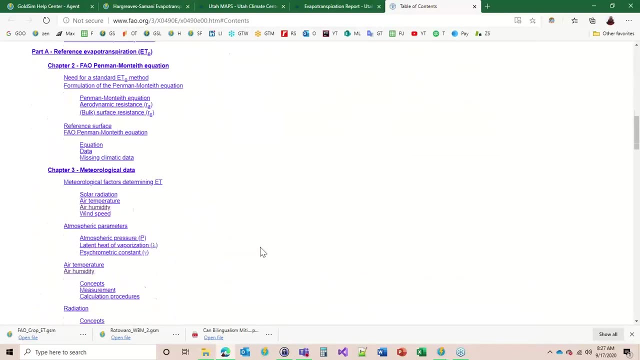 calculations here in a bit, But if you're going to use this, then I highly recommend that you look at the documentation. It's really well written and very thorough. So here it is, And the entire document is online. You can just browse through all of the different. 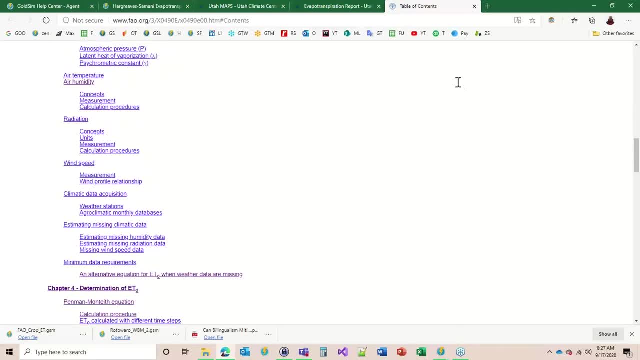 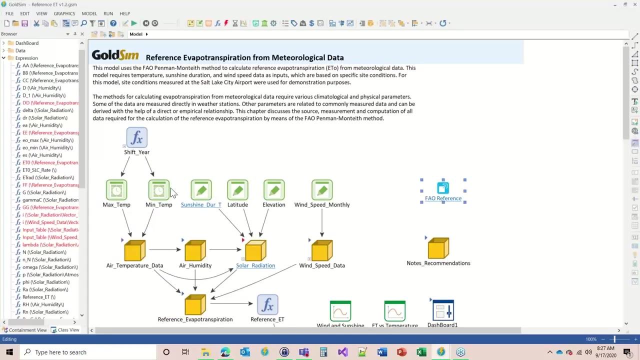 things. You can just browse through all of the different components and read about them, And this is how the model was built. actually was reading this very good documentation, walking through it and putting the equations in. Okay, So with that, then you can see here that this model uses a bit. 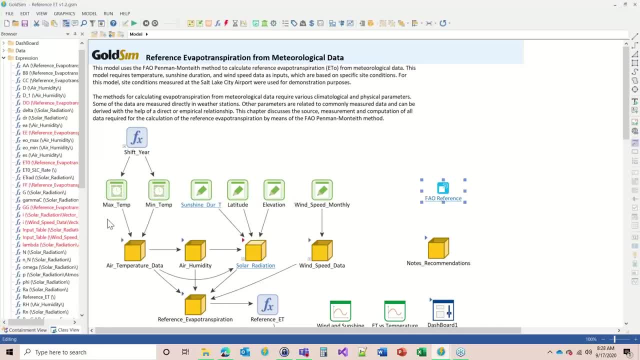